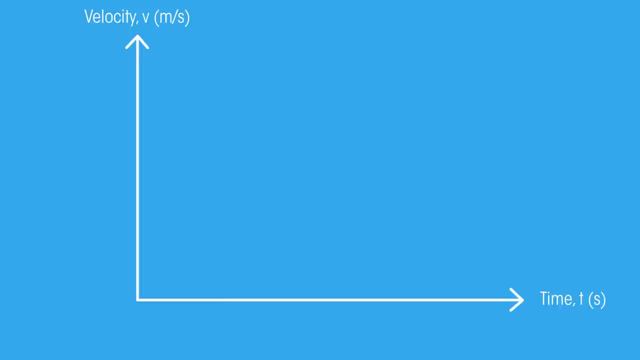 Let's start by looking at a simple velocity time graph To find the area underneath the line. multiply the value on the horizontal axis with the value on the vertical axis. We are multiplying together the velocity of the object and the time it has travelled for. 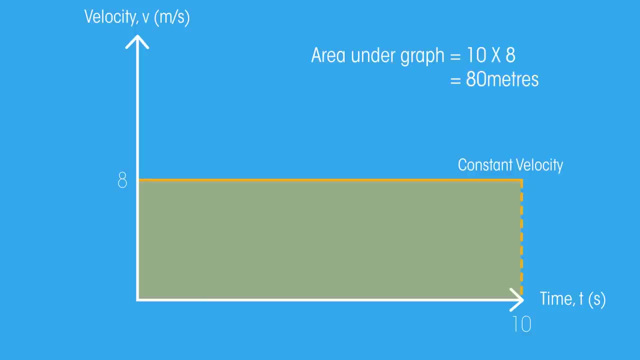 Look at the unit 80 metres. The area underneath the graph gives us the total distance that the object has travelled. So we have velocity, time and distance. The area won't always be quite so simple to calculate. Velocity time graphs more commonly look like this: We can calculate the area underneath the line by cleverly splitting. 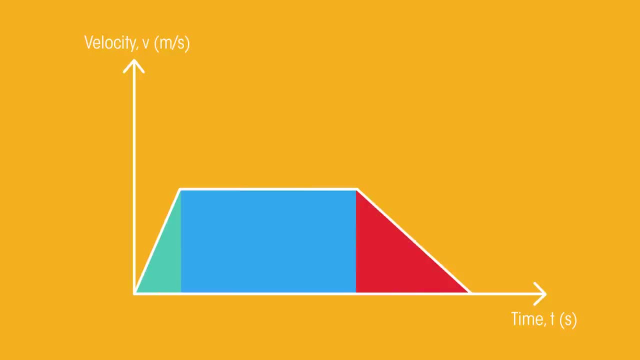 the area into triangles and rectangles. Remember that the area of a triangle is the base multiplied by its height, divided by 2.. Can you work out the distance travelled for this velocity time graph? Work out the total area underneath the graph. Pause the video. 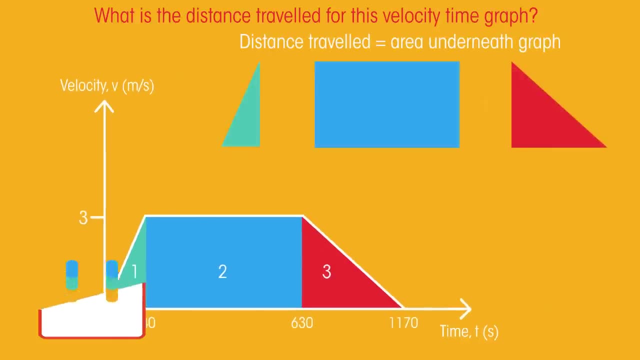 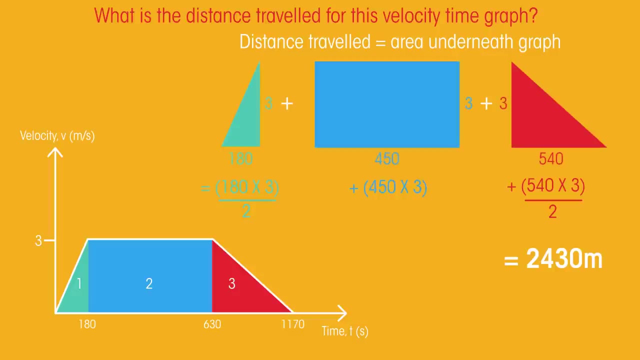 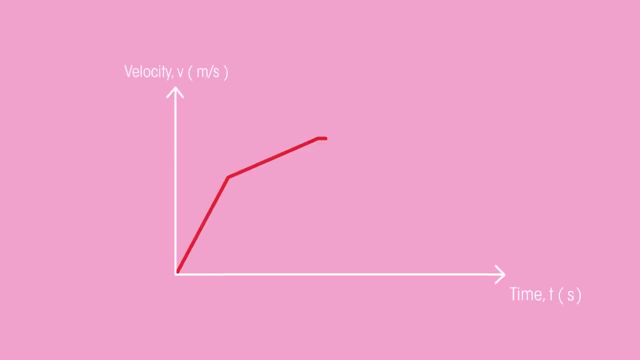 and give it a go. Did you get it right? For most velocity time graphs, splitting up the area will be relatively obvious. However, you might come across some more complicated plots. Splitting up an area like this will be less obvious, Whilst it doesn't matter exactly how you split the area up, the fewer 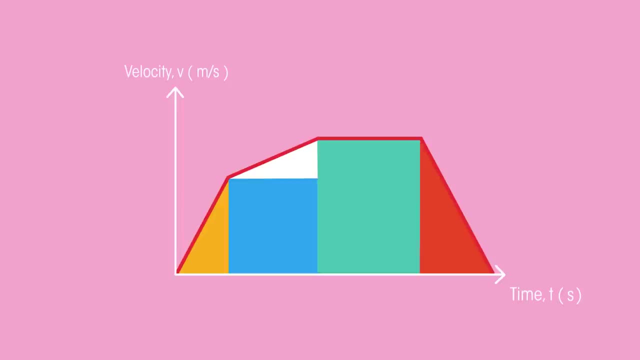 shapes you have, the fewer calculations you'll have to do. As a general tip, try to include a triangle where you see diagonal lines and break it down to a triangle where you see diagonal lines, Or rectangles where there are horizontal sections. Give this one a go yourself. Pause. 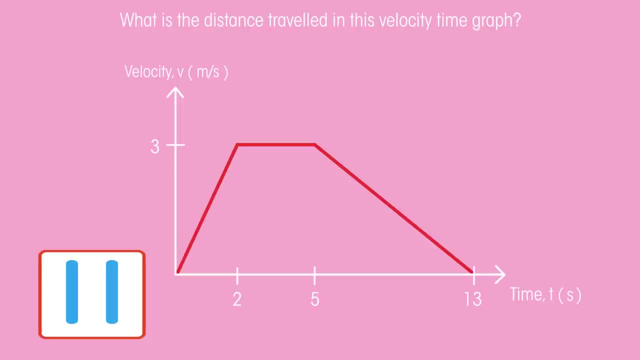 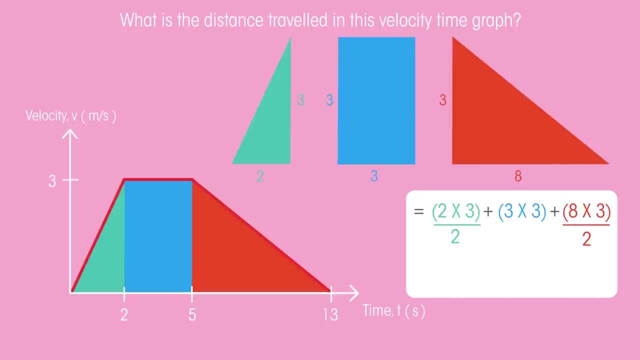 the video and work out the distance travelled. Did you get it right? This means that, for the journey shown by the velocity time graph, the object travelled a total distance of 24 metres. When doing these calculations, just be sure to check the units that you're given, because this will affect what unit you will give in your 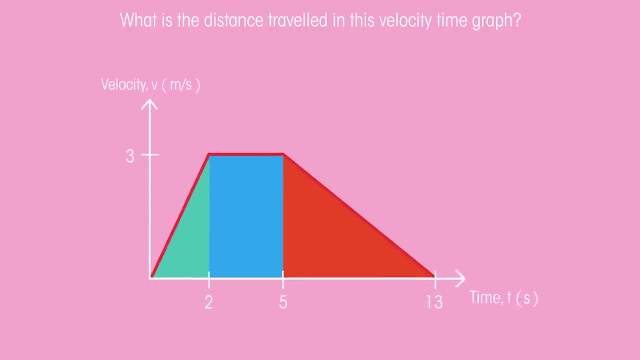 answer for the total distance. For this one it was seconds and metres per second, so the distance in metres is correct. But for this one it's hours and kilometres per hour, so the distance would be measured in kilometres. So there we have velocity time graphs: Velocity on this axis, time on this axis and the area.